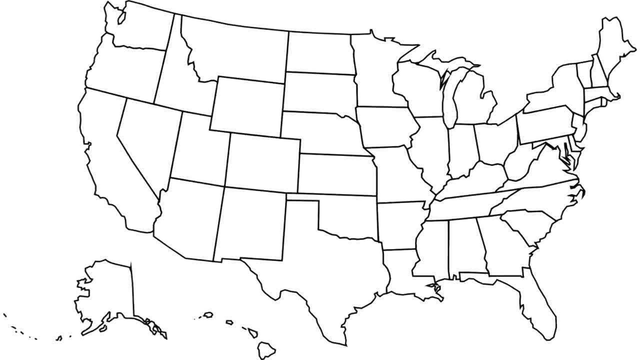 All right, we have a United States map right here. Now, where is the state of North Carolina? Do you know where North Carolina is? Uh-huh, North Carolina is right here on the United States map. The state of North Carolina is in a region of the United States called the Southeast. Uh-huh, the Southeast. 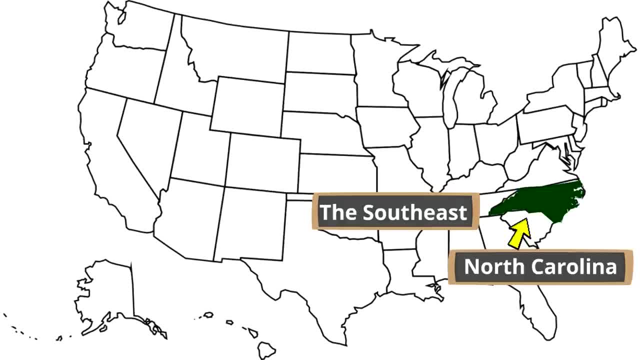 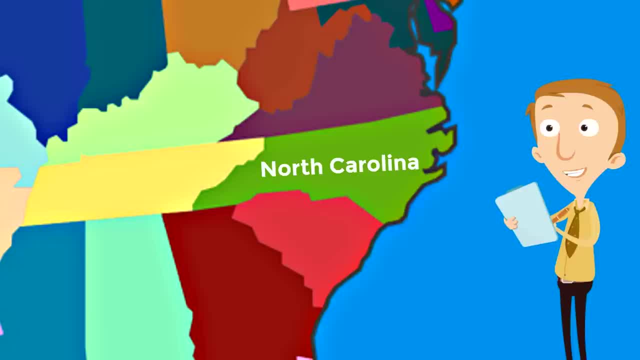 The Southeastern region of the United States. That's really cool. Now we are going to take a few moments to look at the different places that border North Carolina. Bordering North Carolina to the east is a large body of water called the Atlantic Ocean. 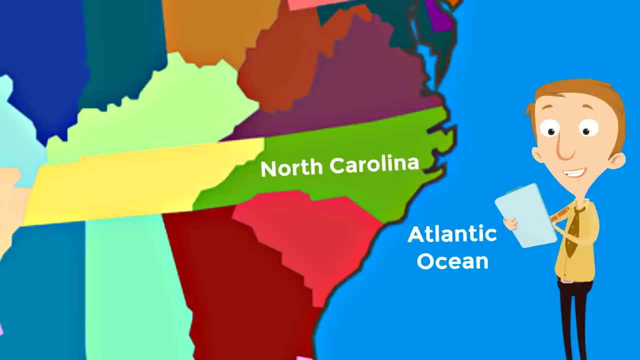 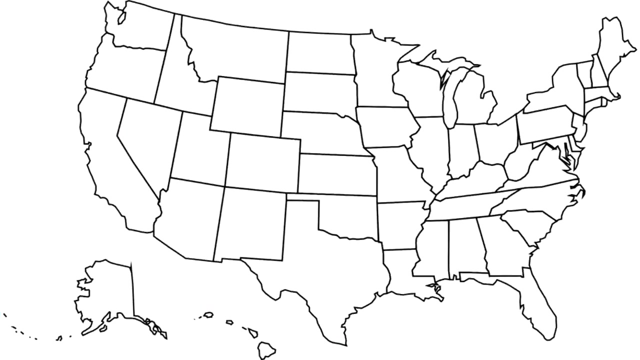 That's right, the Atlantic Ocean. Then bordering North Carolina to the north is the Atlantic Ocean. Then bordering North Carolina to the north is the state of Virginia. Bordering North Carolina to the west is the state of Tennessee. Then there are two states that border North Carolina to the south: Georgia and South Carolina. To review. North Carolina is right here on the United States map, in a region of the United States called the Dome Valley, the South East. Awesome. Now we're gonna learn even more about North Carolina by looking closely at two nicknames that the state has. North Carolina is called the Tar Heel State. 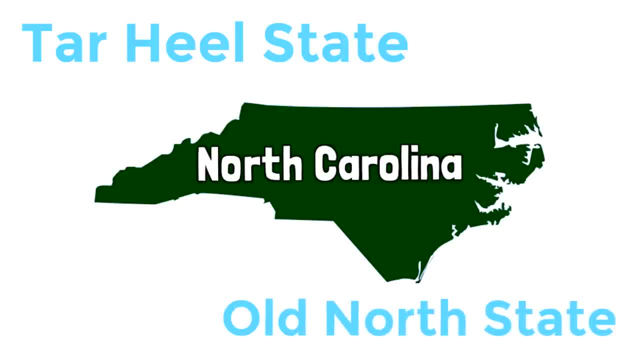 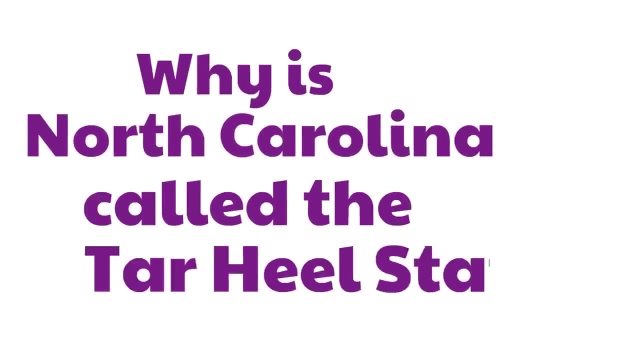 and North Carolina is also called the Old North State. Pretty cool nicknames. First of all, why is North Carolina called the Tar Heel State? Yeah, that's an interesting nickname. Why is North Carolina called the Tar Heel State? Well, there are a lot of pine tree. 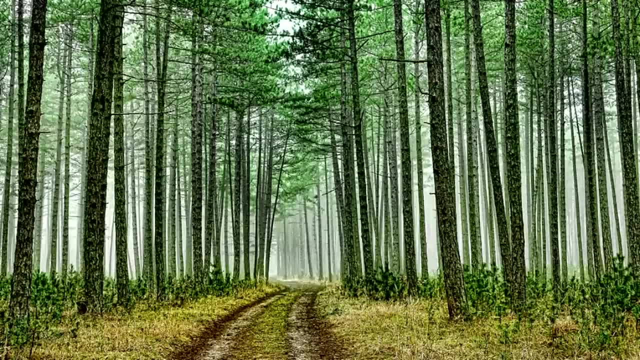 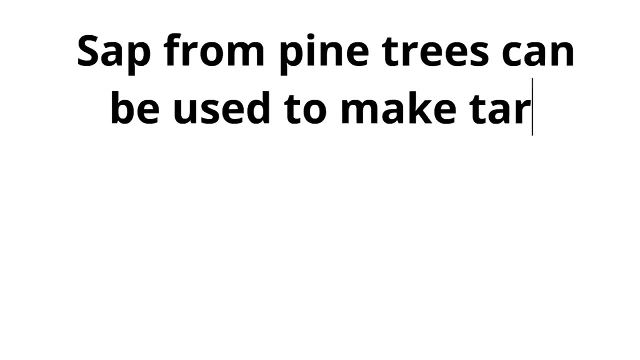 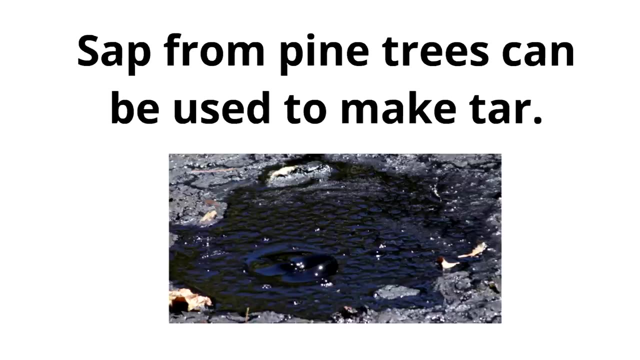 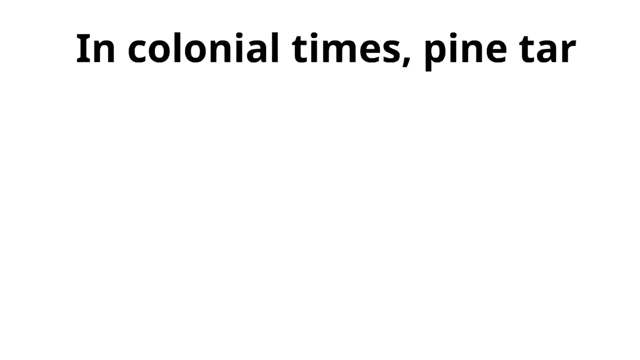 forests in the state of North Carolina. There is a sticky fluid that lives in pine trees and other plants too, called sap. Sap from pine trees can be used to make tar. Tar is a thick, dark, brown or black substance that can be used for many different purposes. In colonial times, pine tar was used in ship. 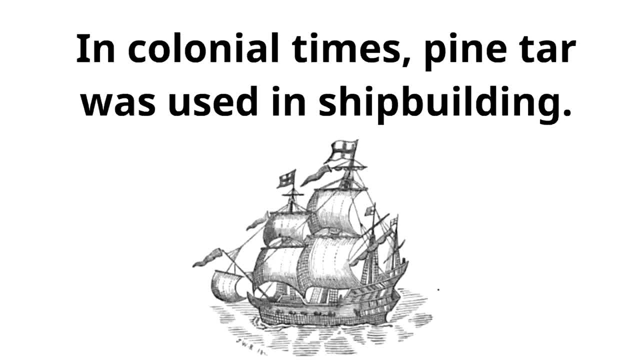 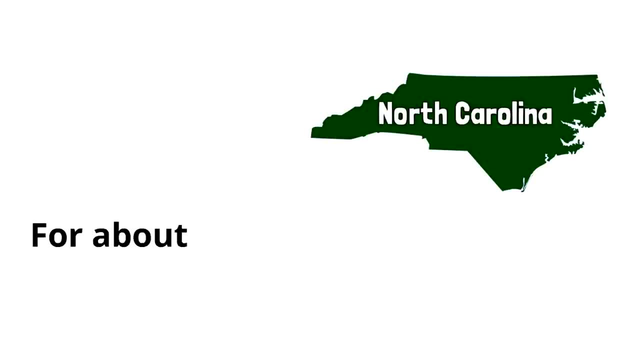 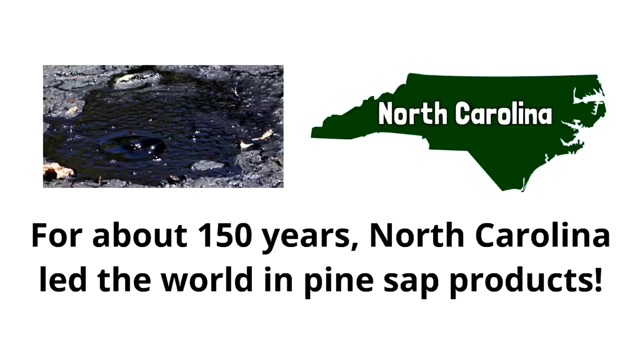 building. You see, the tar would seal the wooden ship so that the wood wouldn't rot in the water. For about 150 years, North Carolina led the world in pine sap products like tar, which is where the name, the Tar Heel State, came from, because there was so much tar that was produced in. 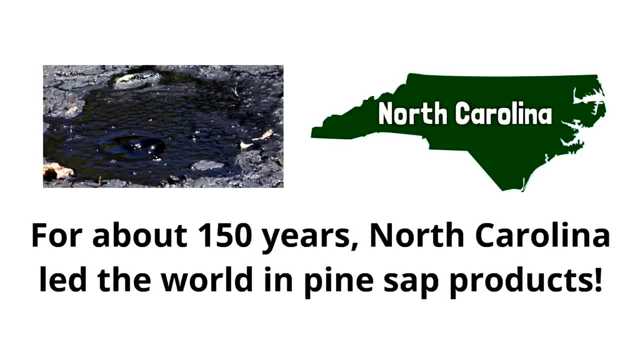 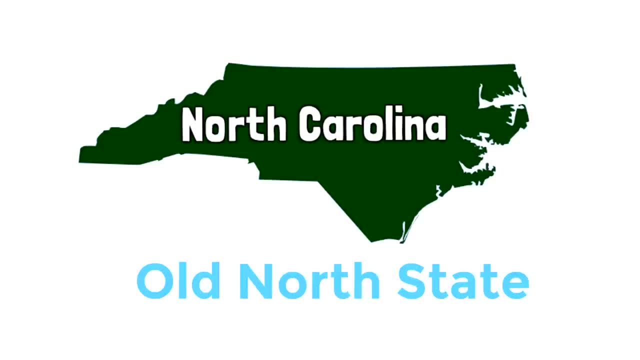 North Carolina from the pine trees- Very cool. Now, why is North Carolina called the Old North State? Well, North Carolina and South Carolina are two different states. They are considered a major part of West Carolina and the world had multiple parall volonties. 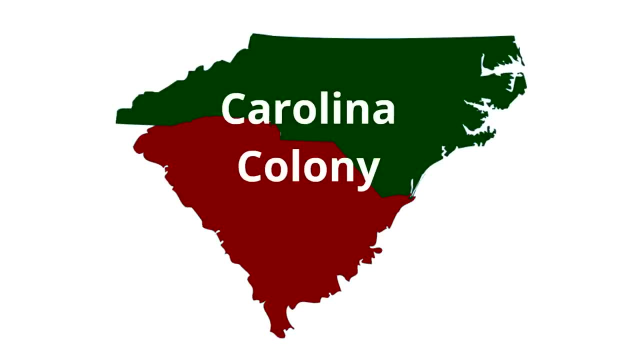 that they are entitled to. North Carolina is one great state. From 1571 until 18acional, the whole Germantown. who was all about dressing up? law enforcement services, adjusts taxes, instant kidnapping, Makkah schönung and other Russian verwandling services? 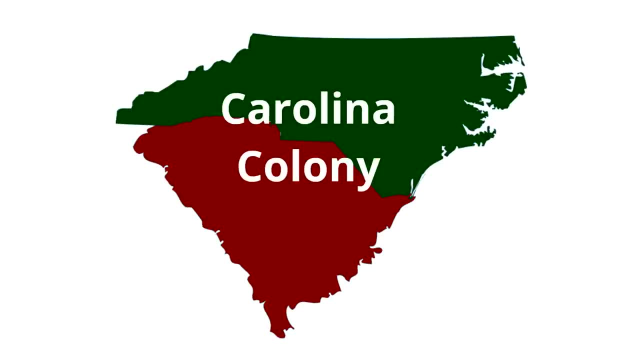 For this people, North Carolina used to be one It use to called Carolina Colony- Not one, It's true, Carolina colony. Then, in 1710, they said: no more of this. Let's split this up. Let's split this. 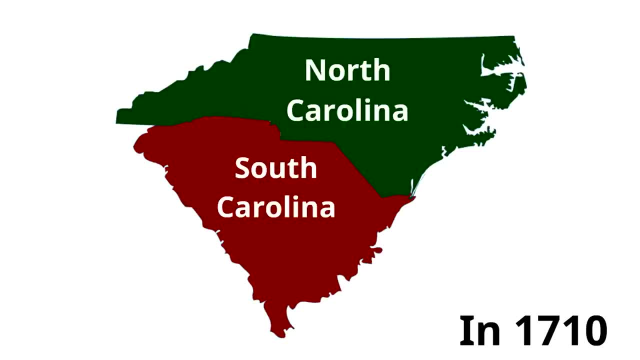 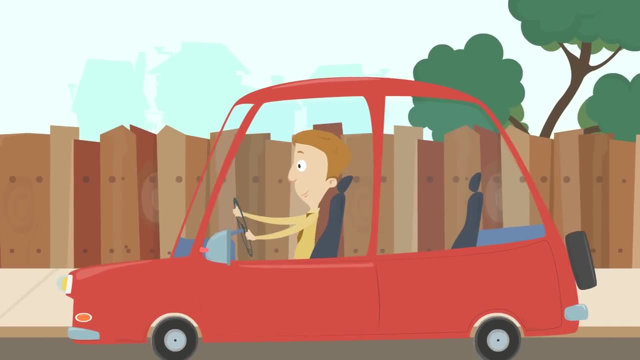 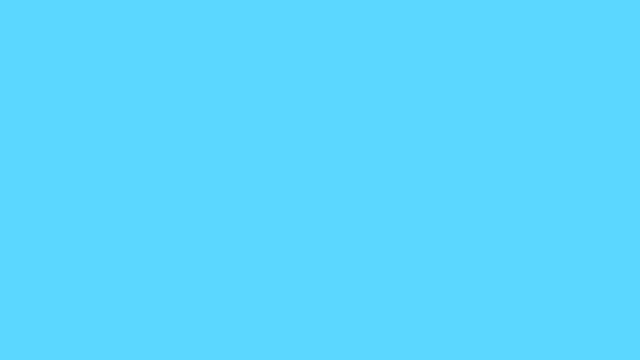 colony up, we'll have North Carolina to the North, South Carolina to the south. North Carolina has been called the Old North state ever since, ever since. okay, now we are going to look at the flag of the Old North State, the Tar Heel State, North Carolina. here is the flag of the state of North Carolina. 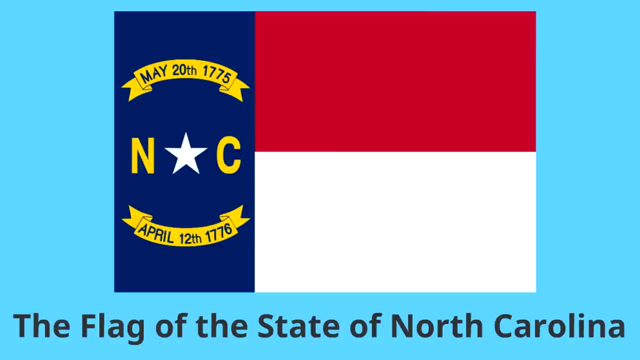 it's a flag that has red, white and blue. in the middle of the blue section is a white star with the letter N on one side in the letter C on the other, representing the initials of the state. and see, there are also two dates that are featured on the flag that are very important to the history of North. 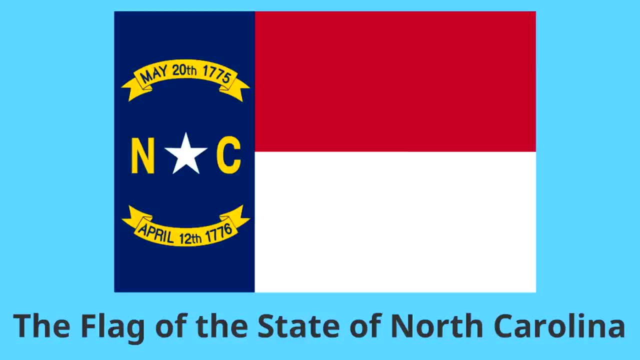 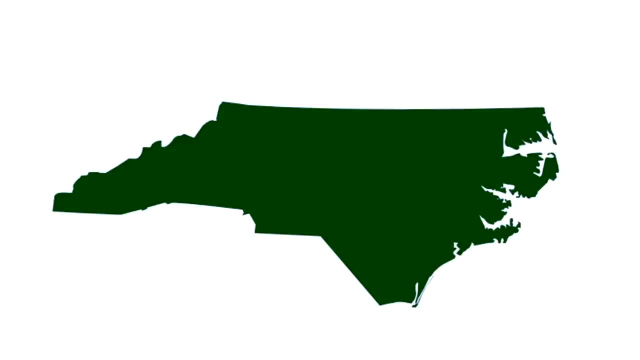 Carolina during the time of the American Revolution. the first was the Mecklenburg Declaration of Independence, signed May 20th 1775, and the Halifax Resolves, signed April 12th 1776. awesome, now we are going to locate two important places on the map of.